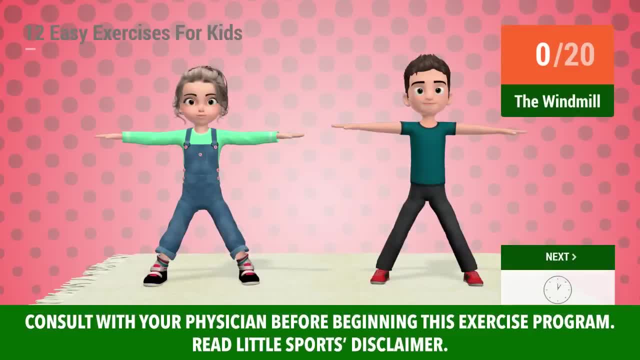 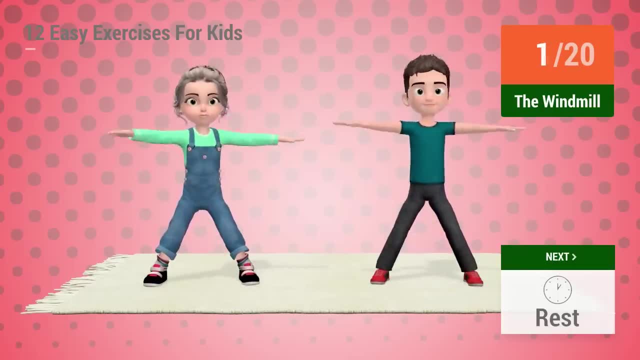 Up next the windmill In 5,, 4,, 3,, 2,, 1, go 1,, 2,, 3,, 4,, 5,, 6,, 7,, 8,, 9,, 10.. 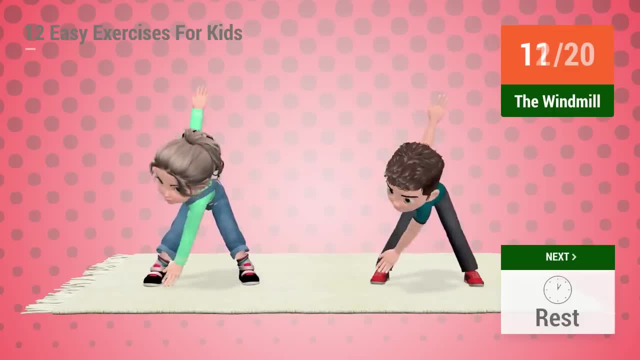 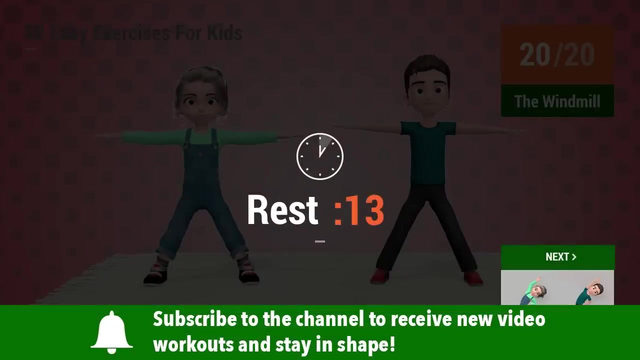 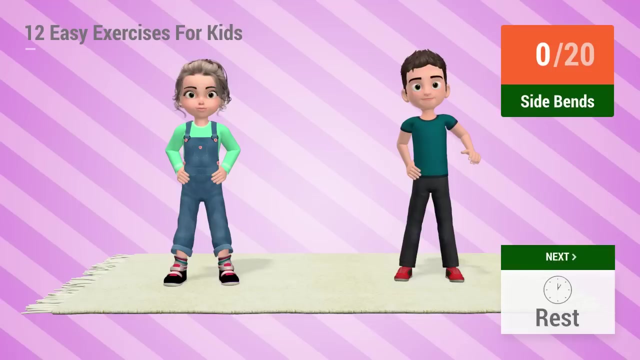 11,, 12,, 13,, 14,, 15,, 16,, 17,, 18,, 19, 20.. Rest time: Up next side bends In 5,, 4,, 3,, 2,, 1, go. 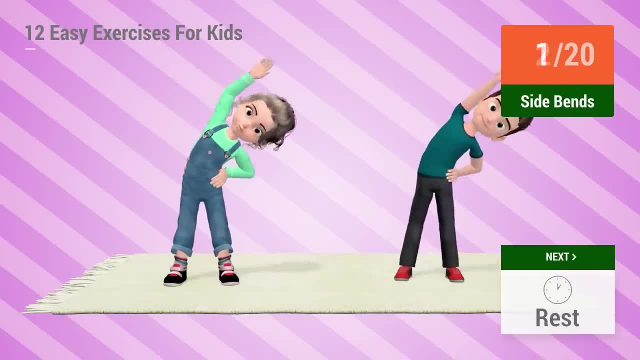 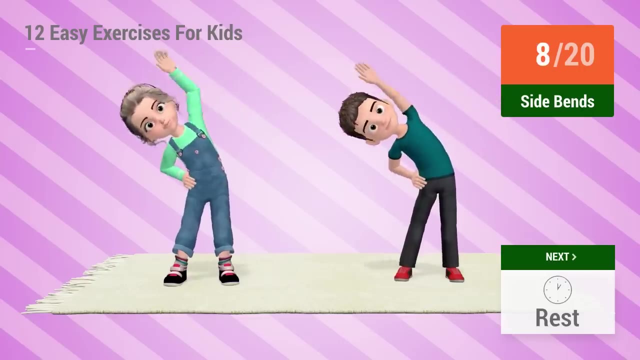 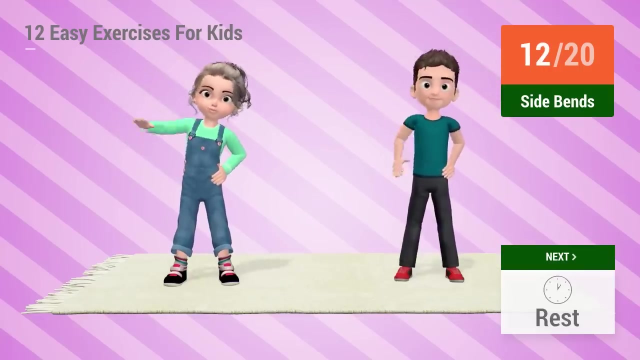 1,, 2,, 3,, 4,, 5,, 6,, 7,, 8,, 9,, 10.. 7,, 8,, 9,, 10,, 11,, 12,, 13,, 14,, 15,, 16,, 17,, 18,, 19, 20.. 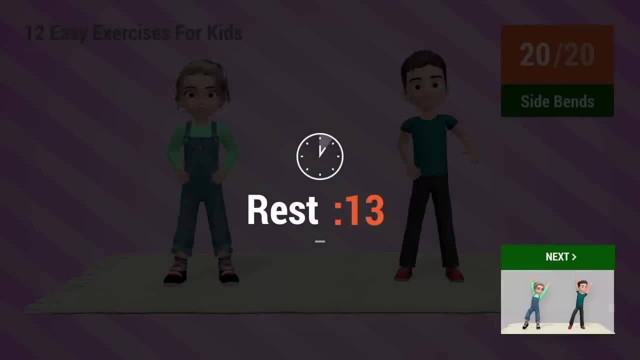 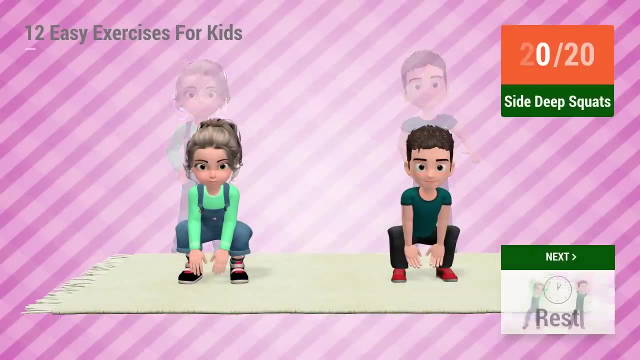 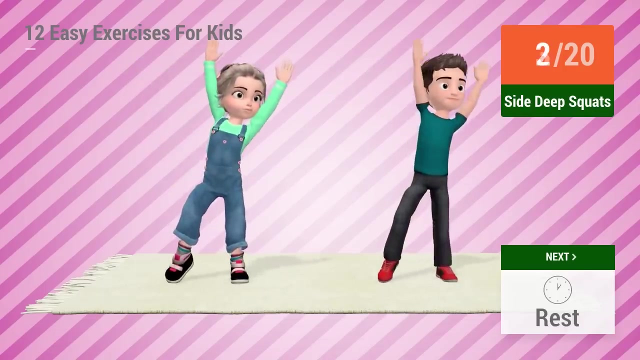 Rest time. Up next side deep squats In 5,, 4,, 3,, 2,, 1, go 1,, 2,, 3,, 4,, 5,, 6,, 7,, 8,, 9,, 10.. 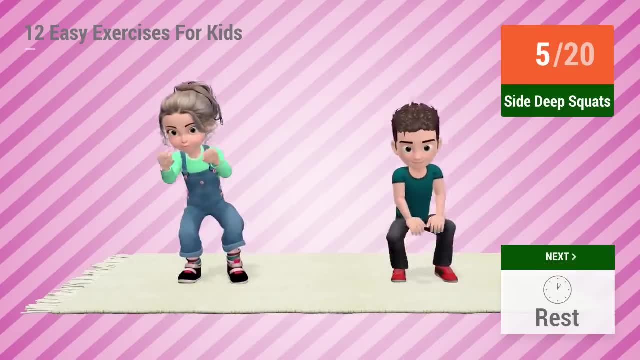 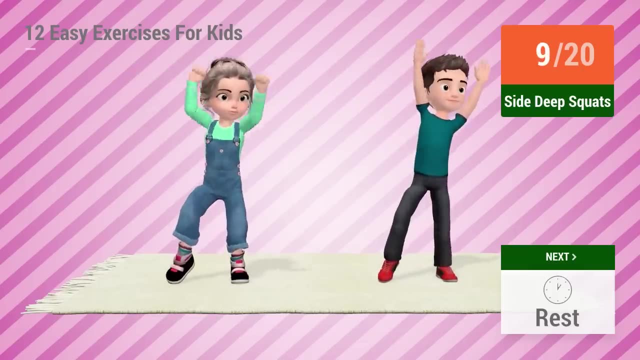 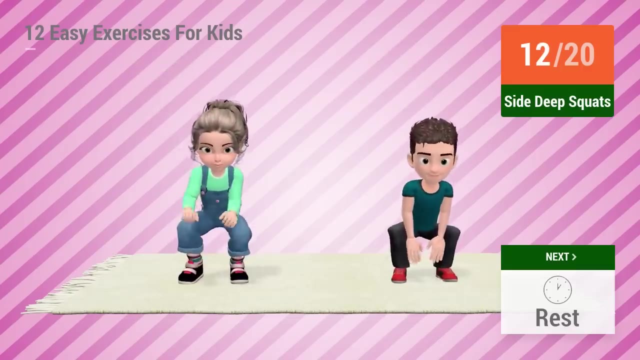 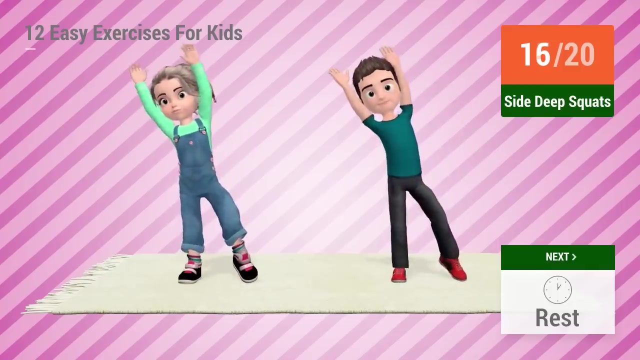 Up next side squats In 5,, 4,, 3,, 2,, 1, go 1,, 2,, 3,, 4,, 5,, 6,, 7,, 8,, 9,, 10,, 11,, 12,, 13,, 14,, 15,, 16,, 17,, 18,, 19, 20.. 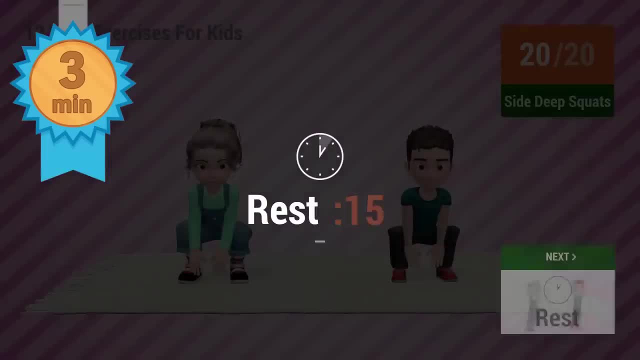 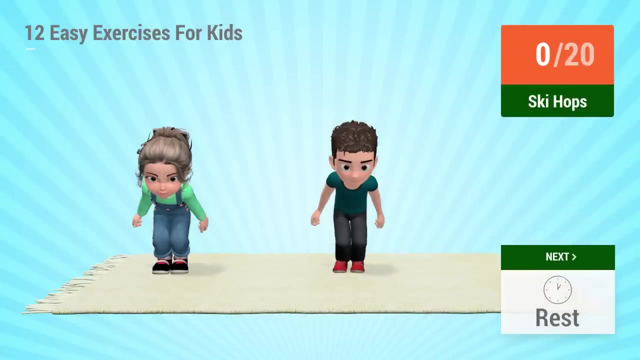 Congratulations, You've passed the 3-minute mark. Keep working out. Let's see how far you can go Up. next, ski hops In 5, 4, 3, 2, 1, go 1, 2, 3, 4, 5, 6, 7,, 8,, 9, 10.. 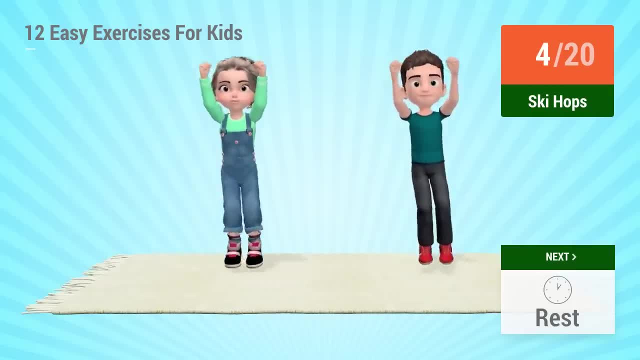 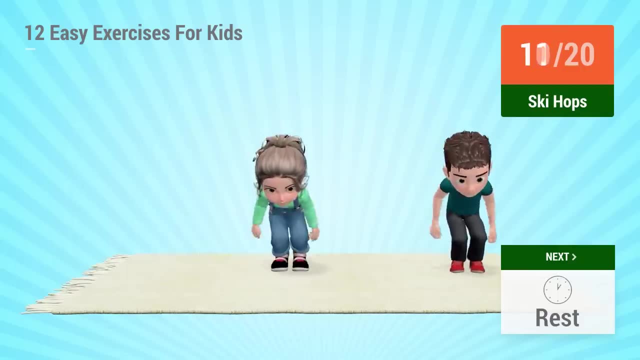 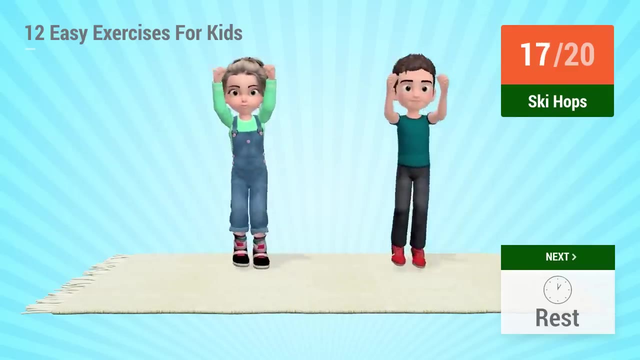 1,, 2,, 3,, 4,, 5,, 6,, 7,, 8,, 9,, 10,, 11,, 12,, 13,, 14,, 15,, 16,, 17,, 18,, 19, 20.. 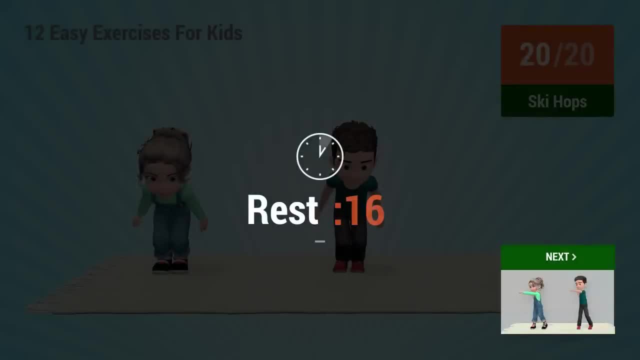 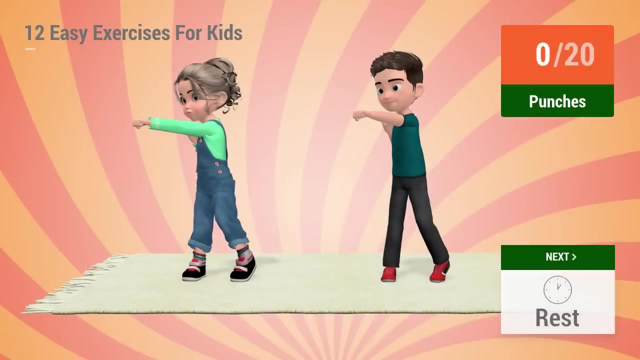 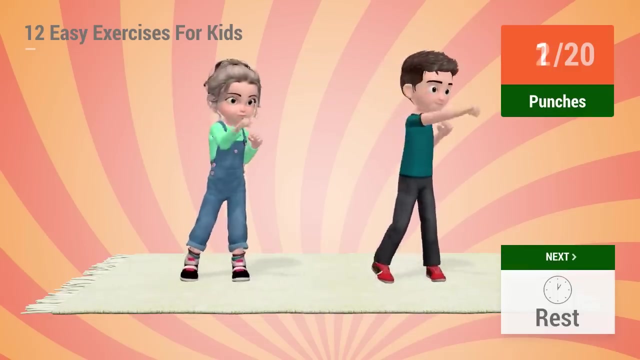 Rest time. Up next push-ups In 5,, 4,, 3,, 2, 1, go 1,, 2,, 3,, 4,, 5,, 6,, 7,, 8,, 9,, 10,, 11,, 12,, 13,, 18,, 19, 20.. 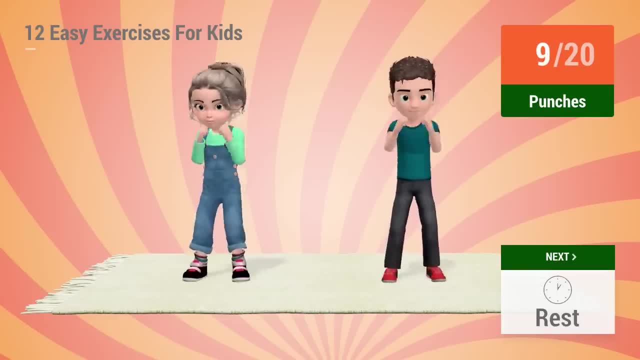 Rest time. Up next ski hops In 5,, 4,, 3,, 2,, 1, go 1,, 2,, 3,, 4,, 5,, 6,, 7,, 8,, 9,, 10,, 11,, 12,, 13,, 14,, 15,, 16,, 17,, 18,, 19, 20.. 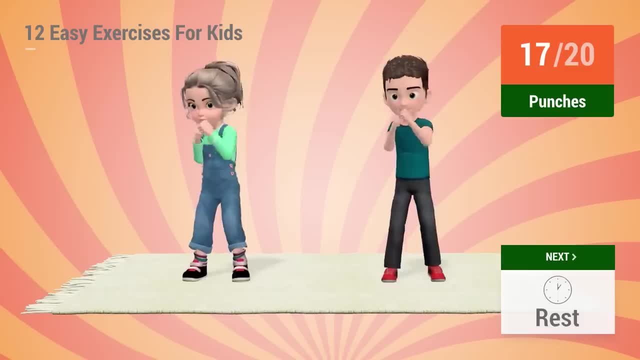 Rest time: 1,, 2,, 3,, 4,, 5,, 6,, 7,, 8,, 9,, 10,, 11,, 12,, 13,, 14,, 15,, 16,, 17,, 18,, 19,, 20.. 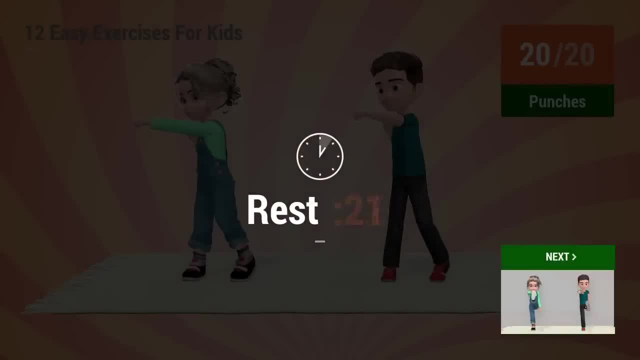 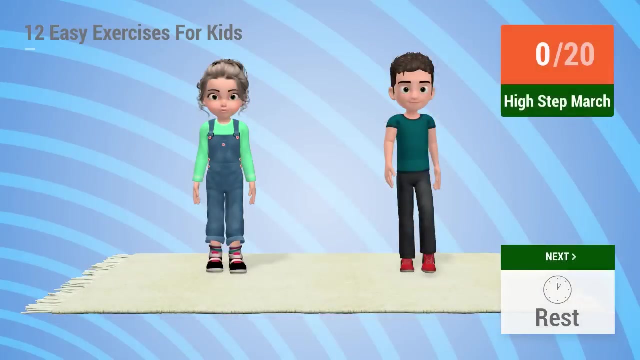 Rest time Up next high step march In 5,, 4,, 3,, 2,, 1, go 1,, 2,, 3,, 4,, 5,, 6,, 7,, 8,, 9,, 10,, 11,, 12,, 13,, 14,, 15,, 16,, 17,, 18,, 19,, 20.. 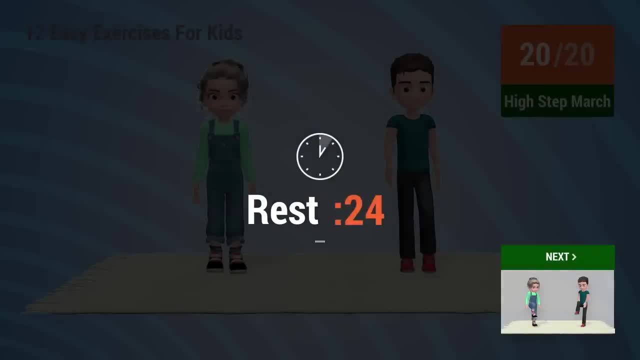 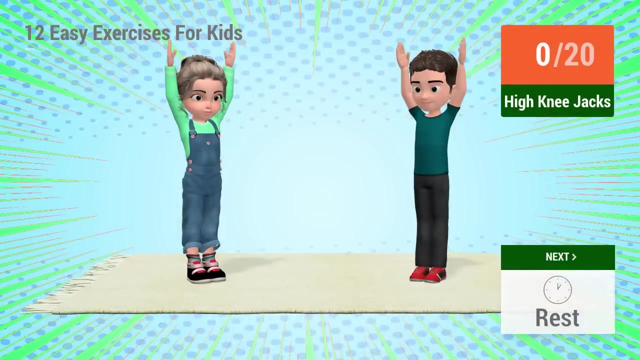 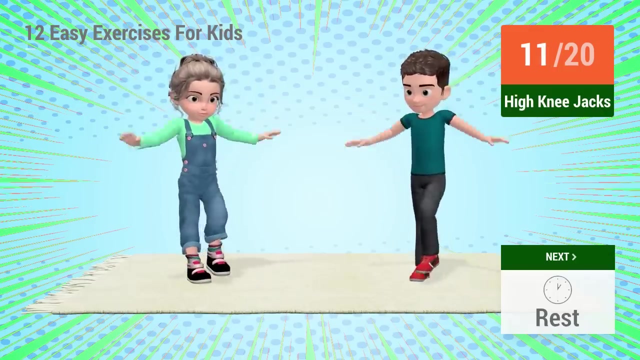 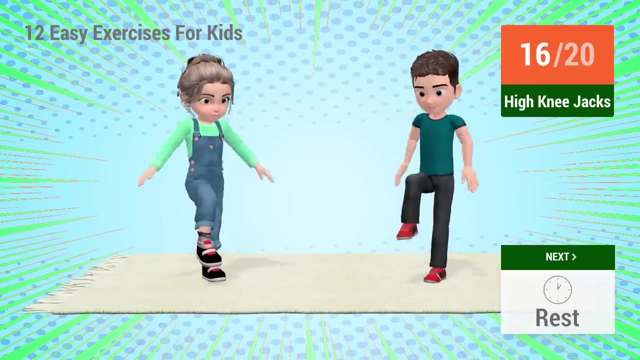 Rest time. Rest time Up next, Up next, Up next. High knee jacks In 5,, 4,, 3,, 2, 1, go 1,, 2,, 3,, 4,, 5,, 6,, 7,, 8,, 9,, 10,, 11,, 12,, 13,, 14,, 15,, 16,, 17,, 18,, 19,, 20.. 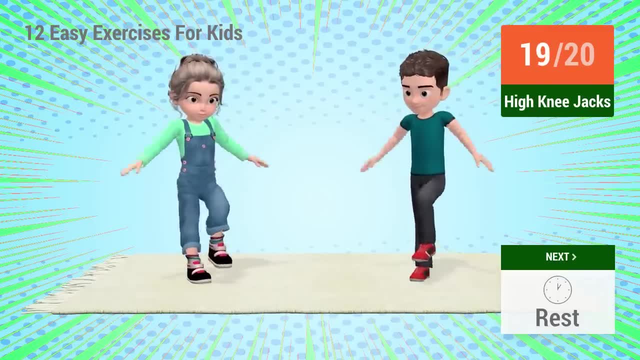 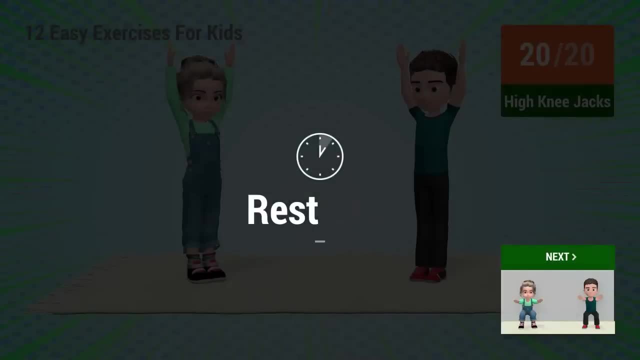 Rest time In 5,, 4,, 3,, 2, 1,. go In 5, 4, 3, 2, 1,. go In 5, 4,, 3,, 2, 1, go. 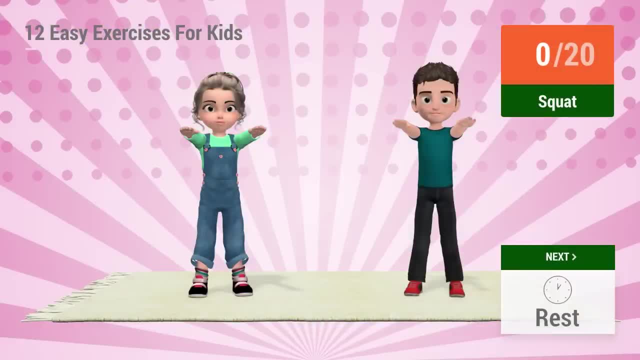 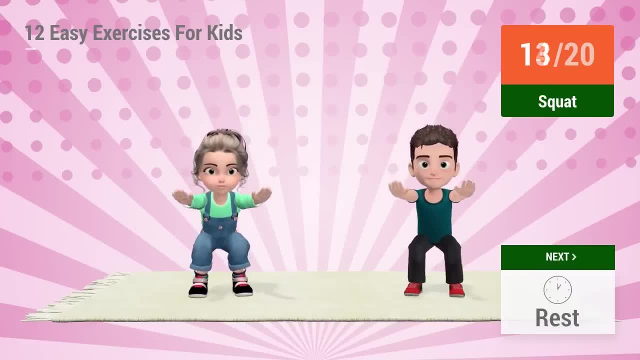 3, 2, 1, go. 3, 2,, 1, go. You got these 8 items, all right. All right, Let's check our остальные Mitras now. 1, 2, 1, go. 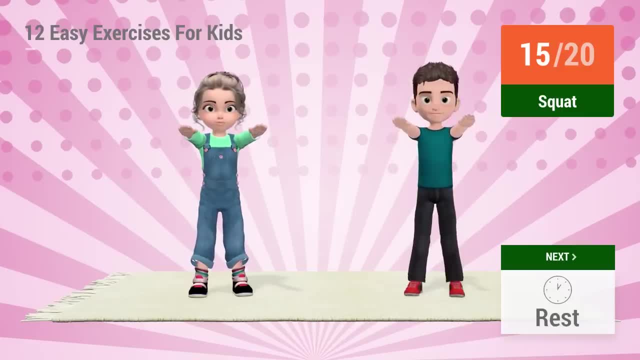 1, 2, 1, go 1, 2, 1, go. 2, 2, 1, go. 5, 2, 1, go. 1, 2, 1, go. 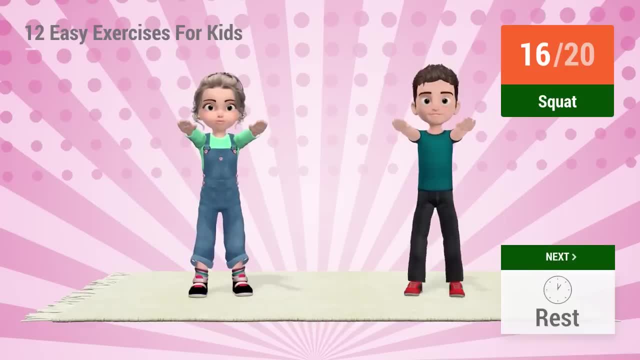 2, 2, 1, go. 1, 2, 1, go. 1, 2, 1, go. 1, 2, 1, go. 3, 2, 1, go. 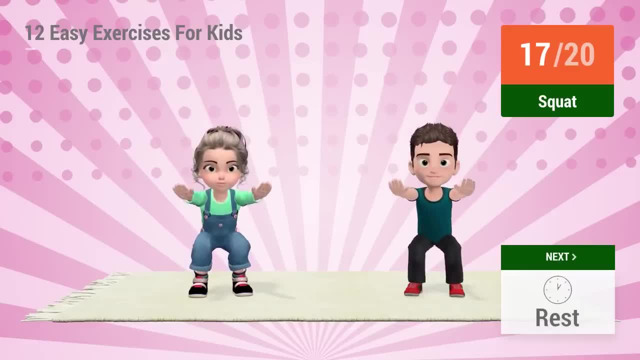 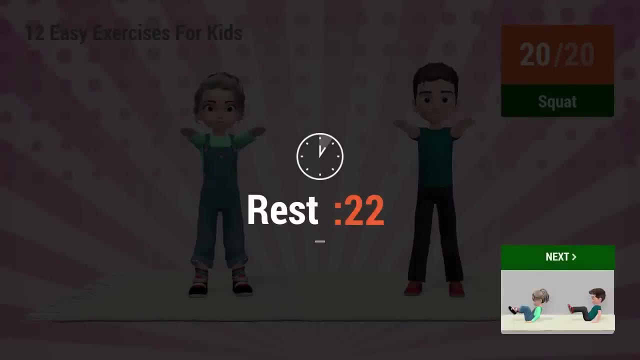 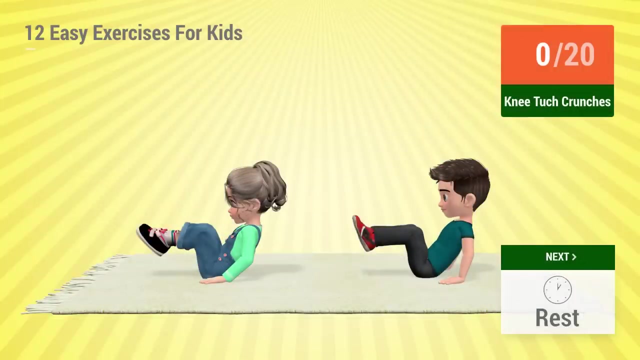 1,, 2,, 1, go, 2,, 3, 1, go. 1,, 2,, 1, go. 18, 19, 20, rest time. up next knee tuck crunches in five, four, three, two, one go. one, two, three, four, five. 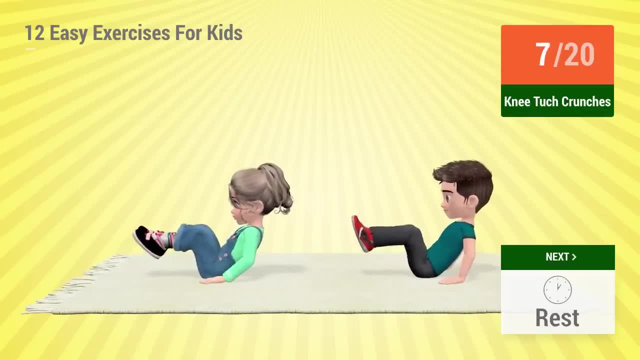 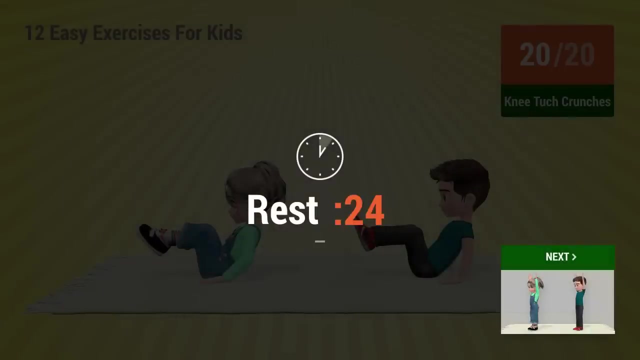 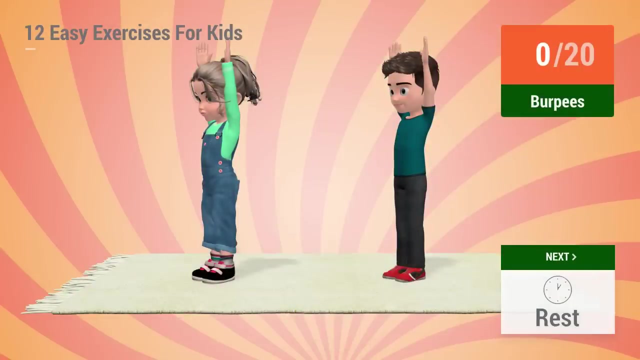 six, seven, eight, nine, ten, eleven, twelve, thirteen, fourteen, fifteen, sixteen, seventeen, eighteen, nineteen, twenty, rest time, time time, rest time, rest, rest, rest, rest, rest time. Up next burpees In 5,, 4,, 3,, 2, 1, go. 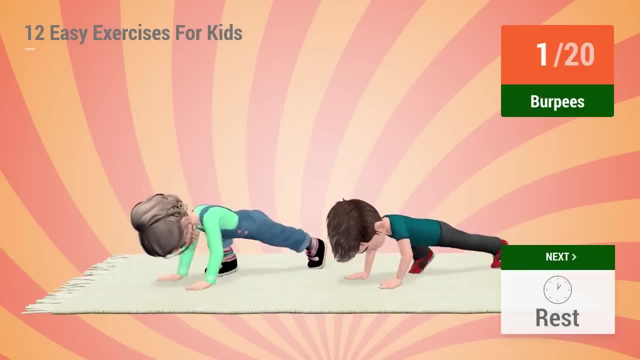 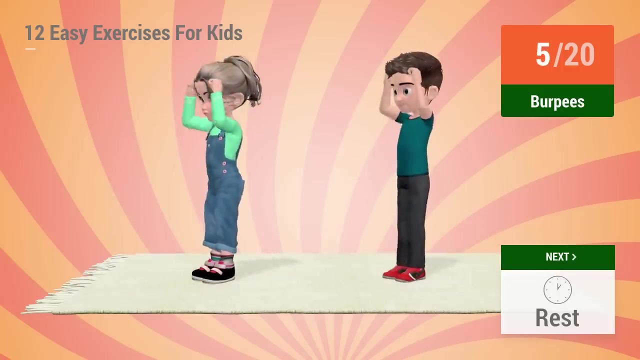 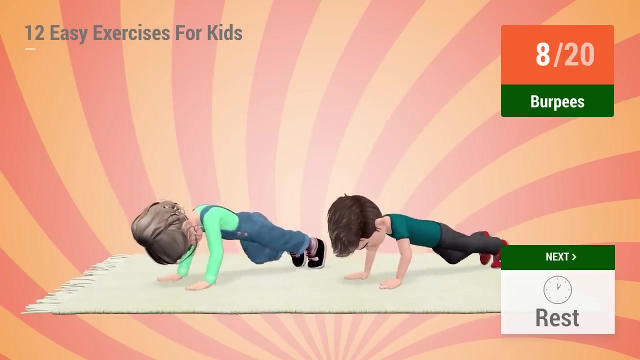 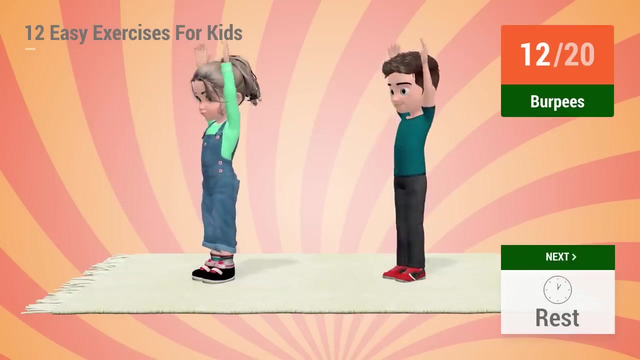 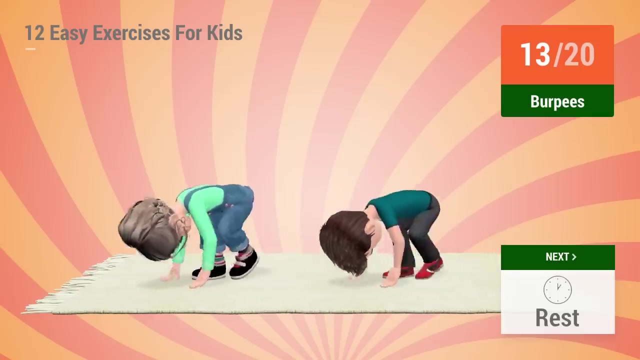 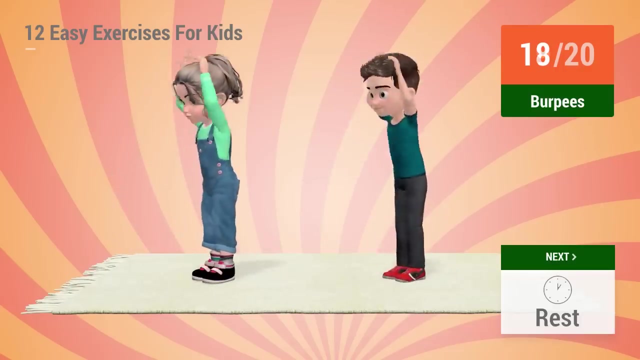 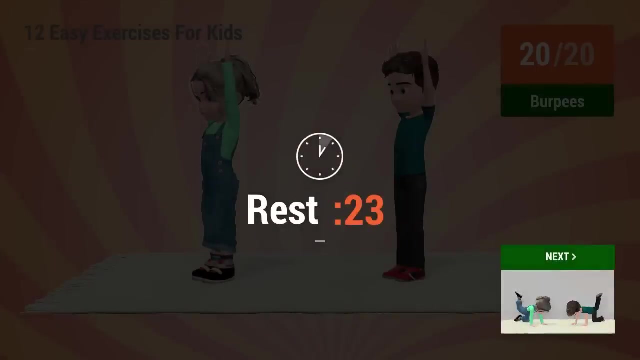 1, 2, 3, 4, 5, 6, 7, 8, 9, 10, 11, 12, 13, 14, 15, 16, 17, 18, 19, 20, Rest time, 21, 22, 23, 24. 25, 26, 27, 28, 29, 30, 31, 32, 33, 34, 35, 36, 37, 38, 39, 40, 41, 42, 43, 44, 45, 46, 47, 48, 49, 50. 51, 52, 53, 54, 55, 56, 57, 58, 59, 60, 61, 62, 63, 63, 64, 65, 66, 67, 68, 69, 70, 71, 72, 73, 73, 74. 74, 75, 76, 77, 78, 78, 79, 80, 81, 82, 83, 84, 85, 86, 87, 88, 89, 90, 91, 92, 93, 93, 94, 95, 96, 97. 97, 97, 98, 99, 100, 100, 100, 96, 100, 100, 150, 15, 60, 60, 61, ше v. 72, 73, 73, 74, 75, 66, 76, 7, 100, 26. 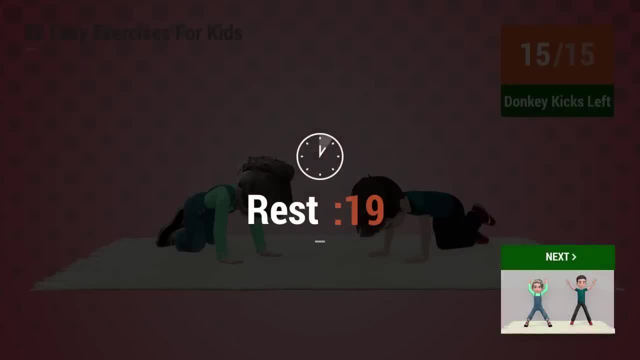 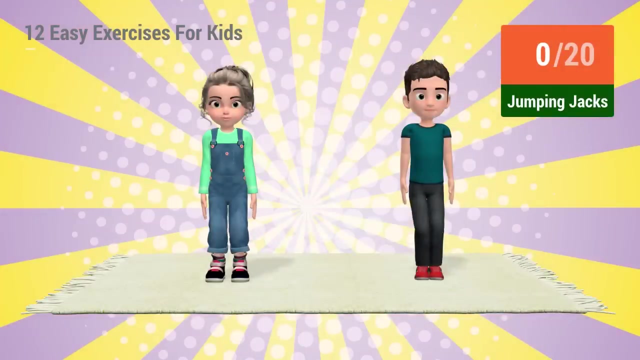 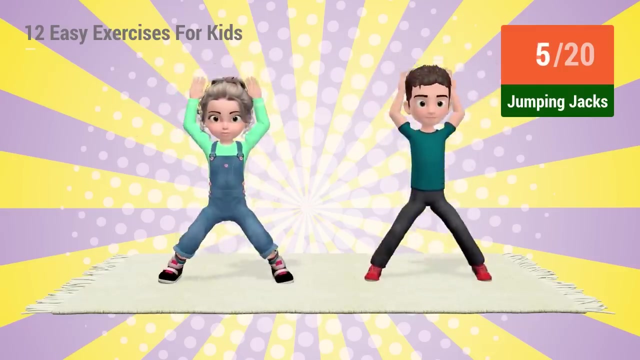 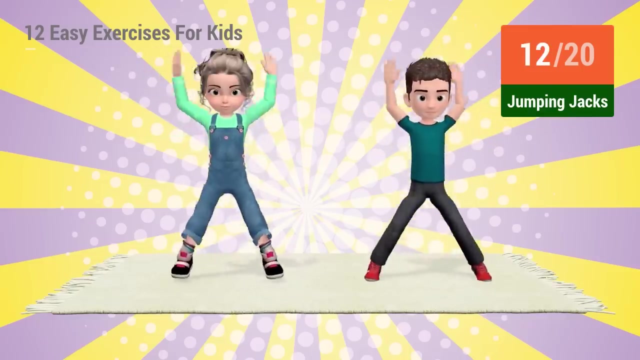 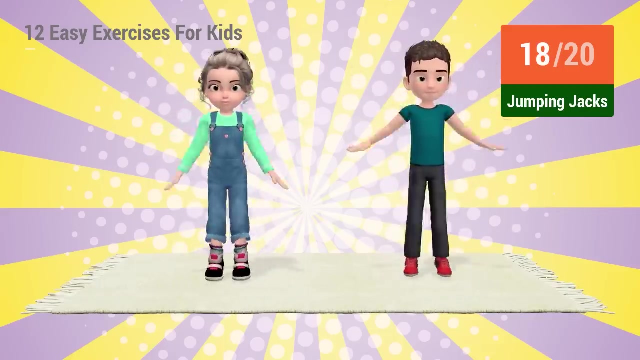 76, 69, 71 為 18. Up next jumping jacks in 5,, 4,, 3,, 2, 1, go 1,, 2,, 3,, 4,, 5,, 6,, 7,, 8,, 9,, 10,, 11,, 12,, 13,, 14,, 15,, 16,, 17,, 18,, 19,, 20. 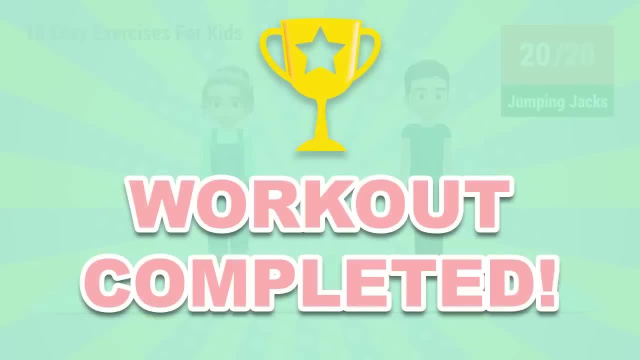 You have successfully completed all the exercises. Good job. Please share this video Work out with people you think should do this workout too.